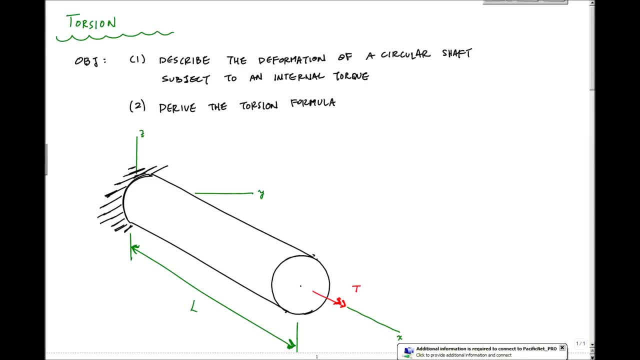 You've created an internal torque in your spinal cord or spinal column so that you can have some muscles that are twisting right. Or taking a piece of chalk and twisted it till failure and seeing the plane of failure that occurs. But in any case, let's take a look at here a solid circular shaft that's subjected to twisting. 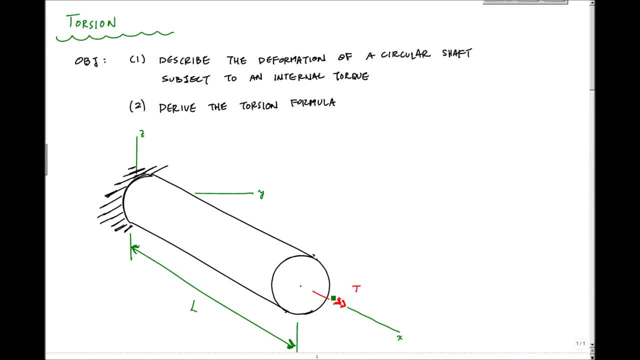 Or this external torque here. Actually, let's make it seem like if I made a cut at this distance L, I would see this internal torque on the inside of that. That would be what's going on on the inside And, as always, this double arrow indicates the direction in which your thumb should go. 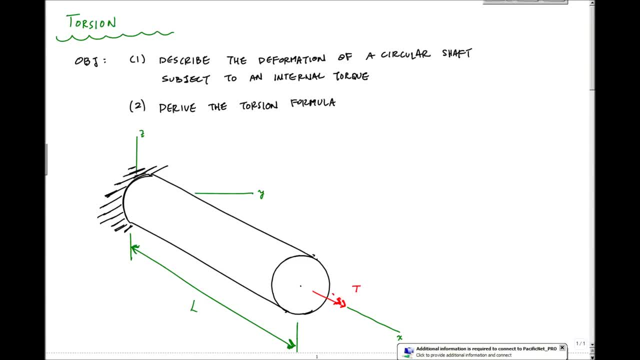 And then the rest of your fingers will curl around in that direction, right there, okay? So here that's indicating the direction of the torque, And just to make sure, just in case There are any questions, Torque is really just another moment. 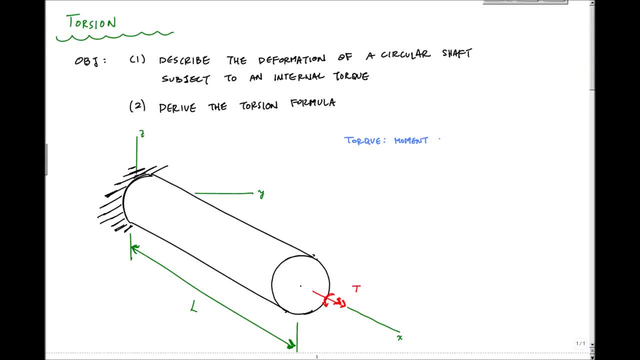 It's a moment that causes twist Moment, causing a twisting action, causing twist Right there. And you know it's no different than any other moment, except you know the moments that you've looked at in 2D are about the out-of-plane axis in 2D. 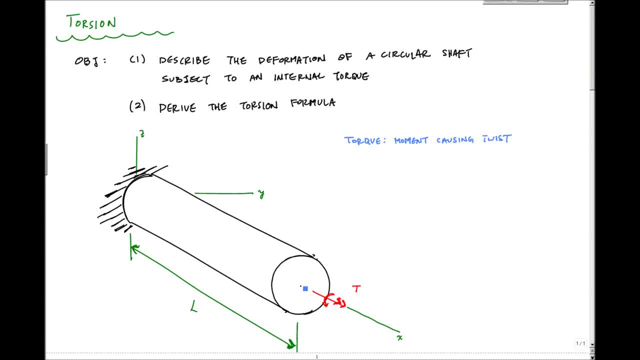 And here, in this case, we're talking about a moment, about the x-axis, which happens to be running through the centroid of the circular shaft. And so, when we apply an external torque, The things you want to know is that the circular cross-sections, the circular sections, 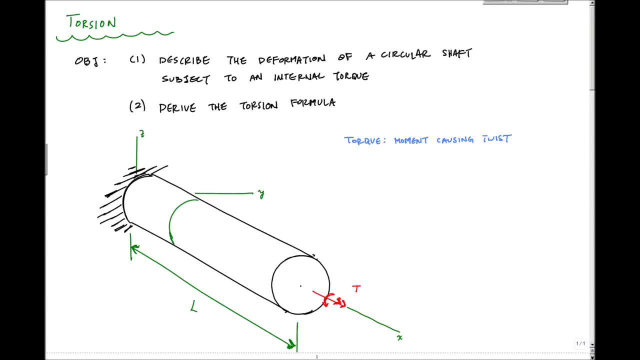 So here let me see if I can draw a circular section right here, Bam, Just using my little. Actually, I have a little tool that I use, Or it's actually not a tool, It's just the inside of a tape. 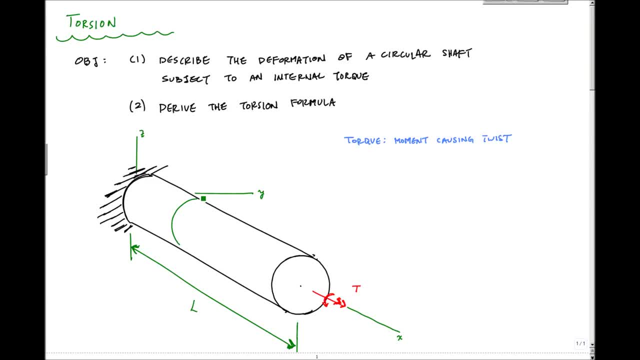 But here bam, to draw my circular sections right here. These circular sections, when you twist something, circles remain circular. So there's no deformation, Remains circular in terms of the cross-section. There's no warping out-of-plane or anything like that. 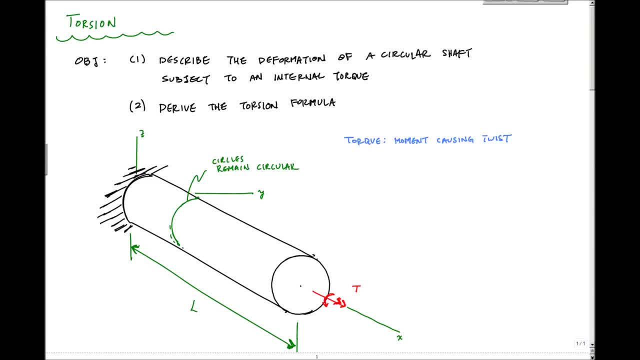 But the thing that does change, the thing that does, is that these lines that are longitudinal at the start of the line- So here let me draw a longitudinal line that's parallel to all this business- Bam, These longitudinal lines twist or they deform. 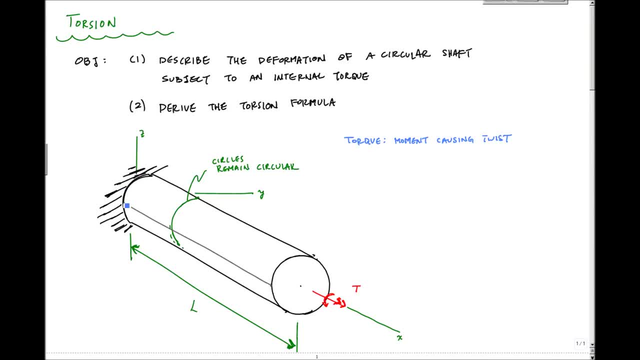 So here, what would happen is, if that line right there, If that gray line, If that gray line, If that gray line was my first line at my under form before loading, then I apply a load to it and I end up with right here some sort of twisting action. 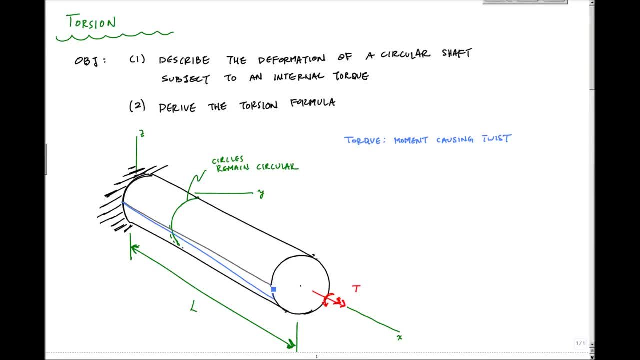 So this gray line turns and rotates and twists right there And, as you can imagine the actual deformation here- because we have a small deformation assumption- the deformation that we would look at or measure is this angle change Right here, that angle change. 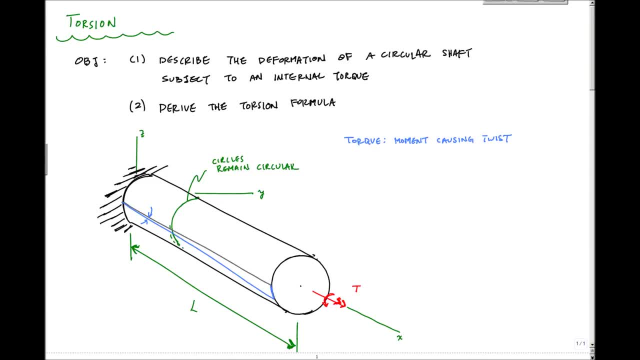 And, as you may have noticed from the strain videos, an angle change, Angle change, is associated with Ding, ding ding. Shear strain Yay, Which means that this torque, internal torque, induces Shear stress. Yes, 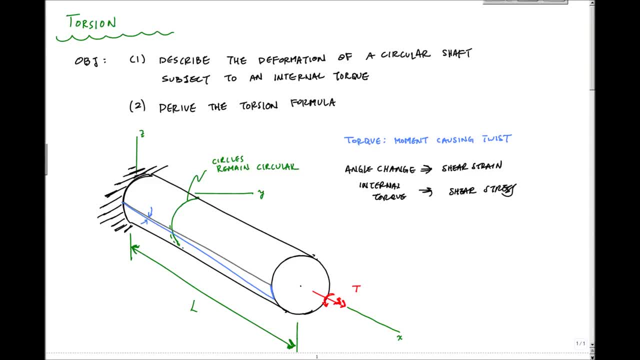 Shear stress, Yeh, Enough the90%. And we will write here this gamma, In fact this angle. right there is a shear strain that's going on And uhm. And another thing to note is that if I look at the crosssection of this, So if I look at my crosssection again, let's start with this gray being my under form line right here- Ooh, got to get that thing in middle right there, Okay. And if that gray right there, Oh, come on, Okay, That gray. 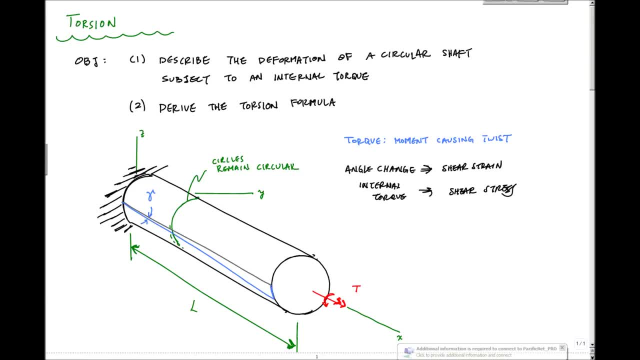 Oh, come on. Okay, That gray a line right here, right through the center of my cross-section. put that dot back there. let's say that's the middle, right there. that deforms to here this position, right here, bam. 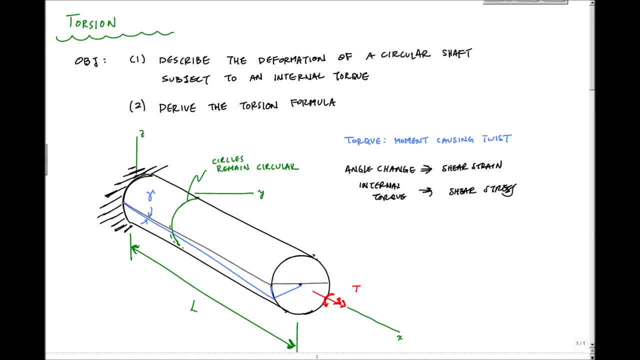 And this angle change right here, which I want to use green just to let you know, that's different than the shear strain- this angle change right here, we'll call that phi. that phi right here is called the angle of twist And in particular in this one, this is the angle of twist at L. 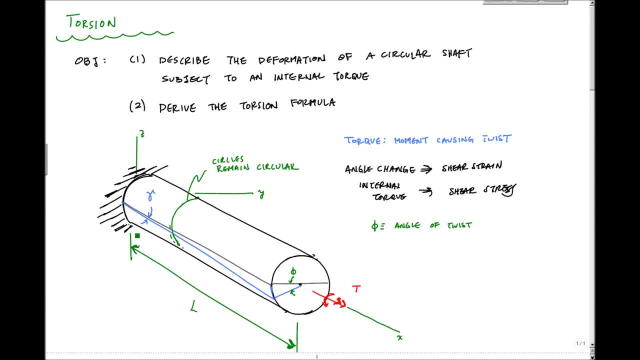 if this is zero, right here along my X axis, this is my angle of twist at L, And if you you can tell from the side view of this line, right here, this angle of twist decreases as I get closer and closer to my fixed angle. 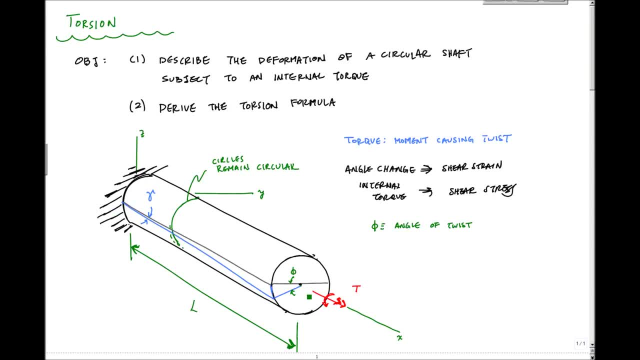 condition right here. so it's a function of this, of a function of the length, or where we are along the length of my circular shaft, using our reasoning of the angle change. here we said that this is associated with shear strain and by you know, knowing that a shear strain, we know that this 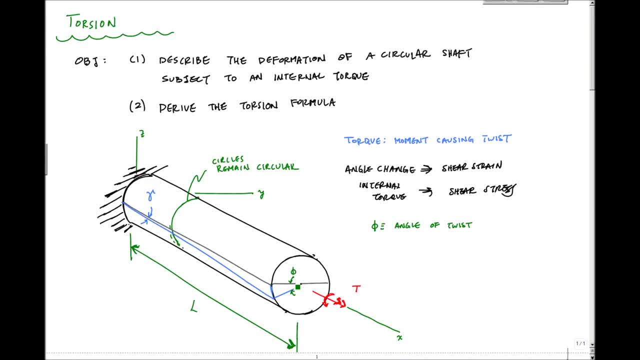 twisting induces a shear stress and that shear stress is on the surface of the circular shaft here. and so if i look at, let's say here, let's say again from this line, right here, i see, let me draw for ourselves. uh, here, let me draw this line all the way across this blue line. 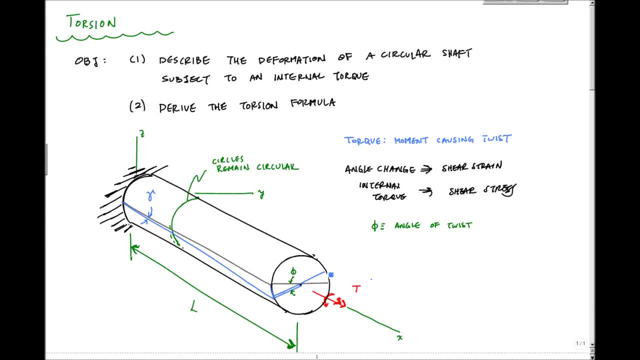 right here, bam, like that, right there, okay, and and so we notice that we have no deformation right here at the center, and then we, as we go out, our deformation, the amount of, or distance from the original to the, the deformed line, if you will, increases, which would tell us that hey. 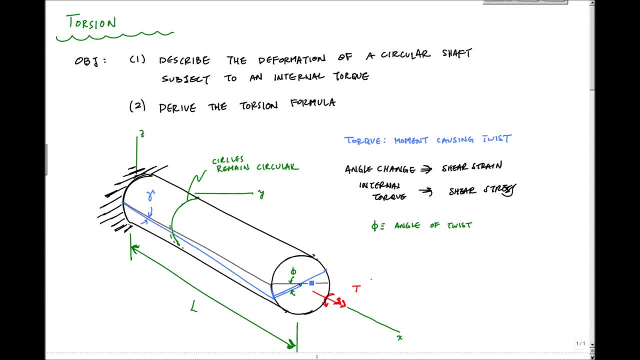 you know what, since our this deformation right here, compared to this line versus this line, is increasing linearly, i would imagine that the stress also increases linearly and and the fact that's true. okay, and so here if i have, for instance, where i have the most deformation, 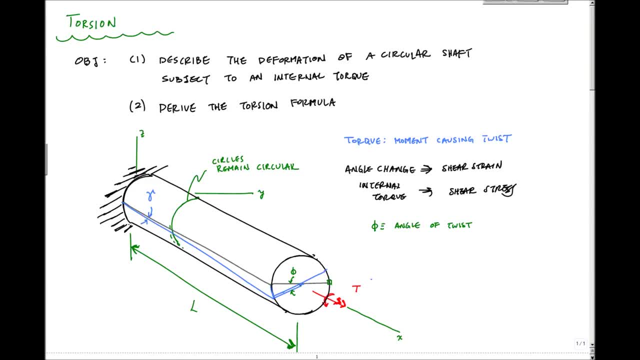 i would anticipate on this little if i could zoom in and i see a little rectangular area on the surface here. this will experience. this location right here will experience the largest shear stress. okay, this will be my tau max and then- and this would be some incremental area- so 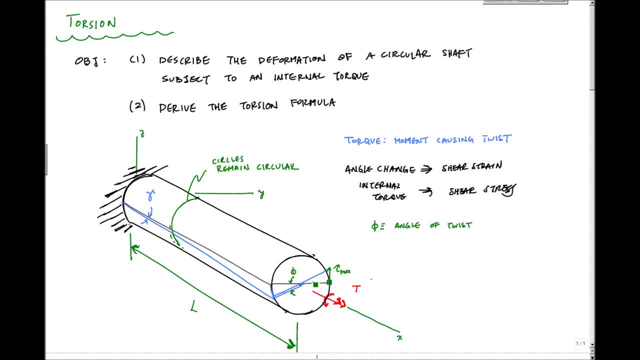 i could say in between, here, along the length or along the radius of this right here, i have some shear stress, which i will denote as tau, acting on this little square area which i will call d a right here and here, if this, if the radius of my shaft. 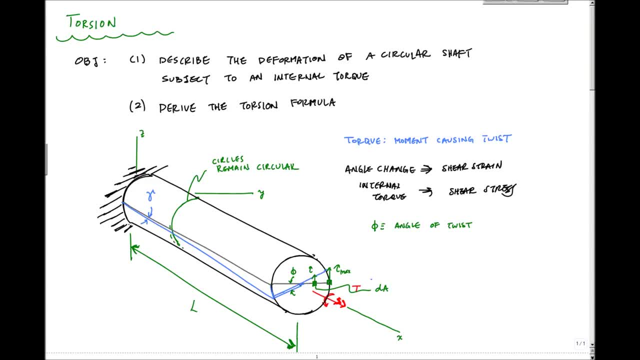 here. let's take the radius. here let's say the radius of the shaft. we'll call that. a lot of your books use the symbol c, so we'll say c is the radius of the shaft, right here. okay, maybe you'd like to use row or r- not row but r, right here- and we'll say: row is the distance to some specific. 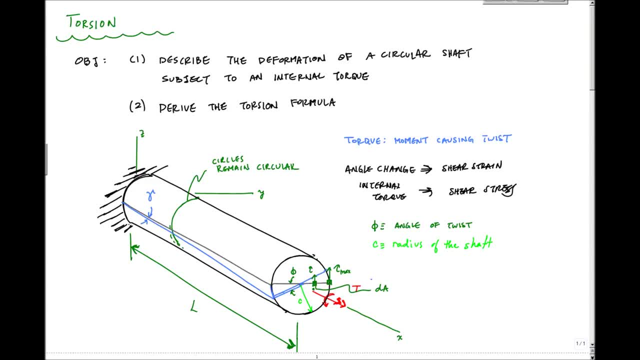 location, some specific, oh don't all right, here we go, row right there, bam row, and i don't even know, but hopefully you can, okay, zoom in on your monitor or whatever, right, and here you've got this, this relationship going on. so we know that this, this stress here, 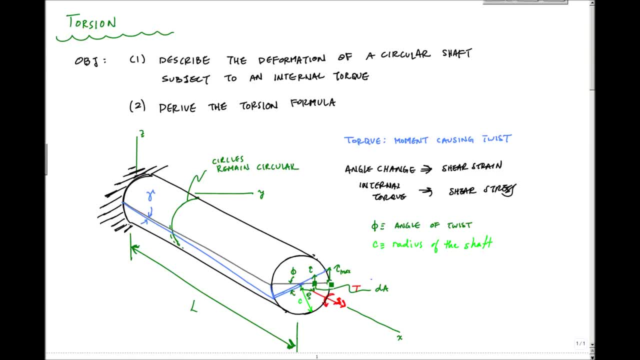 because the deformation, or the ink, the deformation going along the radius from here, where zero deformation at the center line, to the outer edge, where it's the maximum deformation- uh, we know that's varying linearly. so we know we have this intuition or feeling that that, hey, the shear stress. 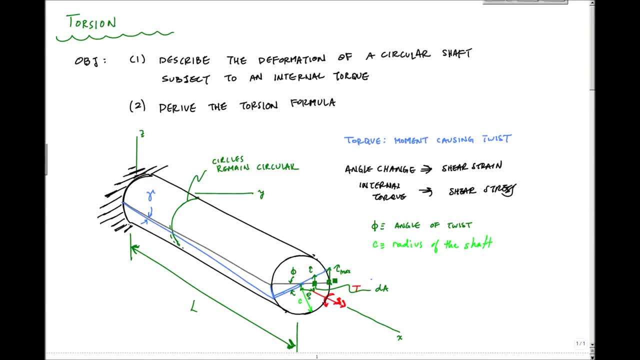 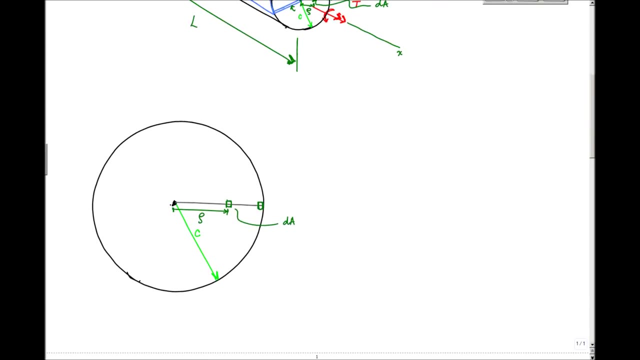 along the face here is also probably varying linearly. okay, so let's take a closer look at this cross section here, and so if i go down, i kind of i just redrew it here. if i look down on this right here, if i zoom in again, just because here at the outer edge is where i experience my largest. 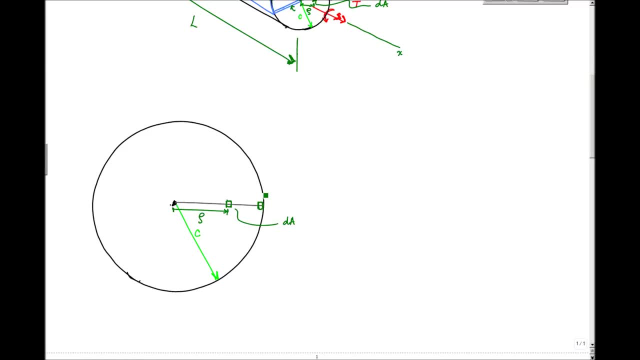 deformation i anticipate having here and i'll use a towel for stress or use red right here, the shear stress on this little incremental area, right here here i anticipate it's saying it's at the very outer edge, tau max right here at the very outer edge, a distance c from the, from the center here, a radial distance c, i expect, the tau max or maximum. 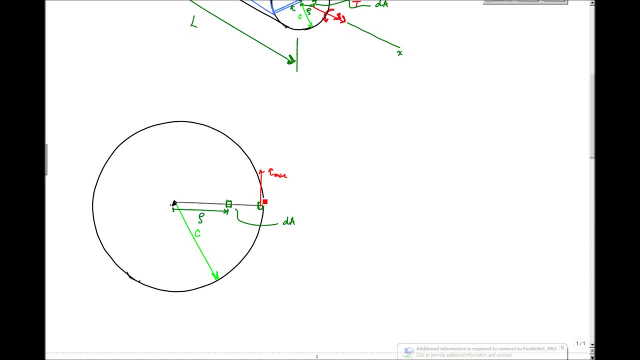 shear stress and i anticipate this all the way around the entire cross section. okay, on the outer edge is my maximum shear stress and then here, if i take an arbitrary location or arbitrary radial distance from the center, here i know that i'm going to have some sort of linear relationship. 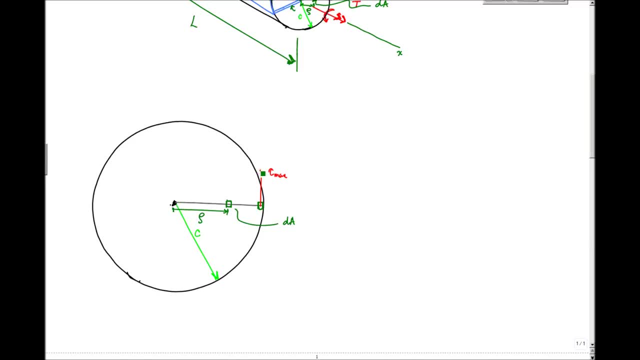 okay, because my deformation is also linear. i know my stress is also linear because hook's law is linear. okay, and so here i have, bam, some stress, some shear stress on this increment area, some arbitrary radial distance row away. so here i'll call that tau, and i know that the two i can relate. 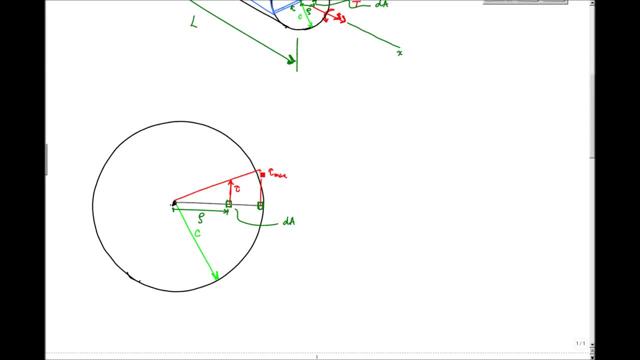 the two by similar triangles. um, um, um. by similar triangles. this relationship would be tau: max over c is equal to the shear stress at any arbitrary location divided by the radial distance to that location from the center, and it doesn't matter which line on the cross section i look at. so 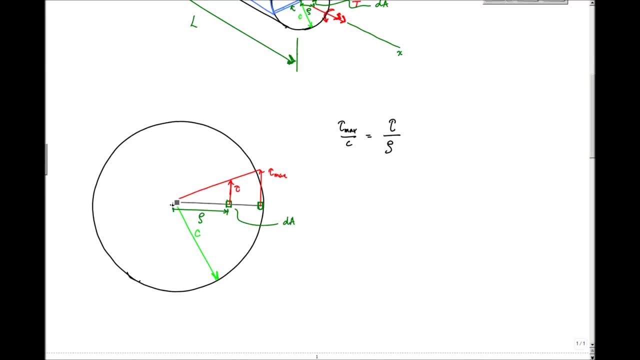 even if i were looking at some arbitrary line at this angle, right here, my stress profile, my shear stress profile is the same, right because it's also again, no matter what line i'm looking at, i have a linear distribution or linear deformation going from the center out towards the outer radius. 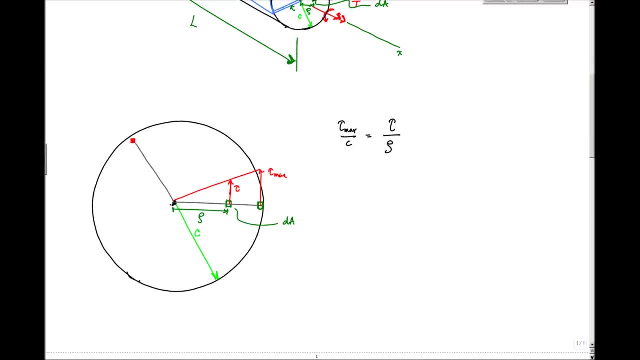 and i'm going to experience here, we'll call this tau max and then as well like this: and it doesn't matter what line i'm going to have there, if this is my some location right here and this is my distance row as well, this would be again an arbitrary. 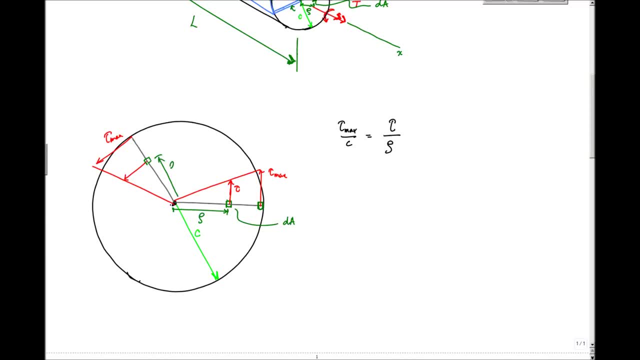 distance row away from my center, right here, intermediate, if you will acting on this line here. what we are assuming is that this was a sort of shiseFF by reproducing my. This internal torque has to be equal to the sum of all the shear stresses DA times rho because we have – this is a torque right. 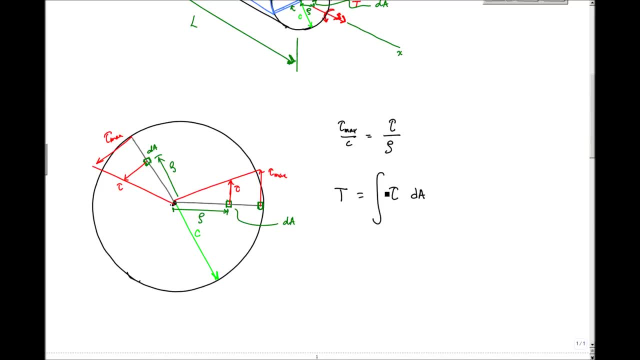 Force times – so tau times. DA is going to give us a force, and then we need an arm or a distance, so we'll have this rho And then, if I – and this DA, just to make sure, is really a double integral in maybe like polar coordinates or something that you would have to resolve if you want to calculate this without the help of some other things that we're going to have, 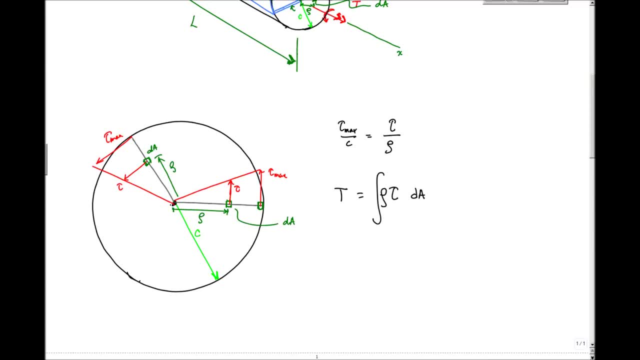 But here, for instance, let's substitute now this definition of the shear stress, tau, which is tau is equal to rho times tau max divided by C. And if I substitute that for tau over here, then I would get that the torque. The torque is equal to – let's see, I'll group the rows together so I'll say tau max over C times rho squared DA. 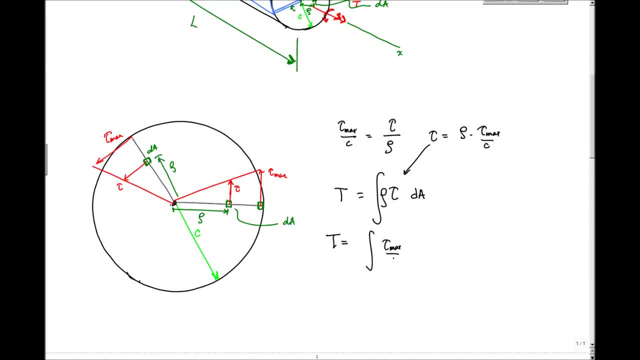 And in this case, tau max is a specific value at the very end or at the outer radius or outer edge of my shaft, And C is also the outer edge, It's just the radius. These are all constants, And so this becomes this: tau max over C is rho squared DA.